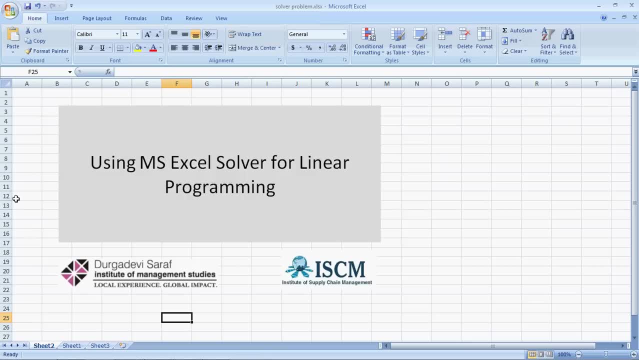 Hi, We will learn how to use Microsoft Excel Solver for linear programming based optimization problems. Solver makes linear programming very easy. You can forget the difficult, simplex methods and the graphical methods. Solver takes care of the mathematical part of linear programming. To be able to use Solver, we need to ensure that the Solver add-in has been installed. 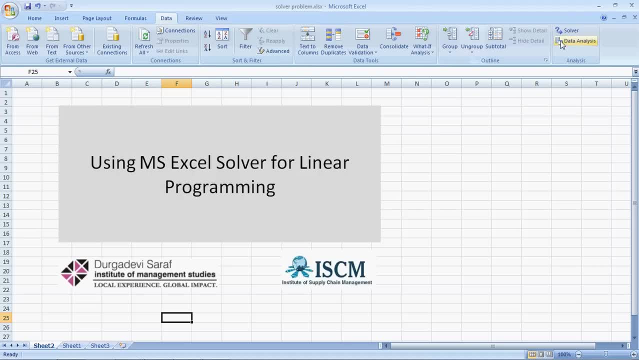 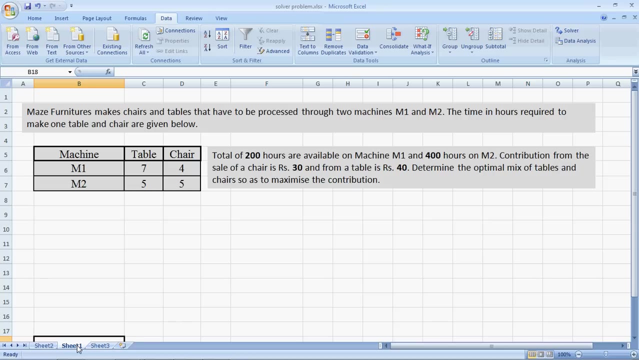 Have a look at the Data tab at the top. You should see the Solver add-in. In case you do not see it, you might have to get it installed Now. let's have a look at this problem: Maze Furniture. They make chairs and tables that have to be processed through two machines, M1 and M2.. 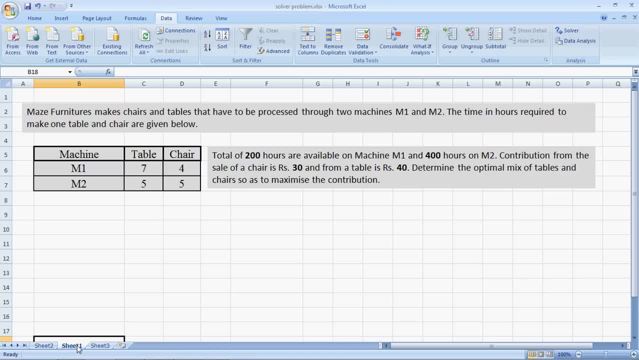 The time in hours required to make one table and one chair are given below. A table takes 7 hours on M1 and 5 hours on M2.. A chair takes 4 hours on M1 and 5 hours on M2.. A total of 200 hours are available on machine M1 and 400 hours on M2.. 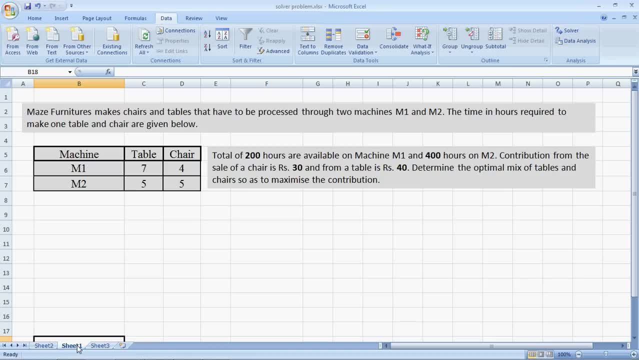 Contribution from the sale of a chair is Rs 30 and from a table is Rs 40. We need to decide the optimal mix of tables and chairs so as the maximum contribution is received To solve this problem. we need to understand that this is a classical and simple linear programming problem. 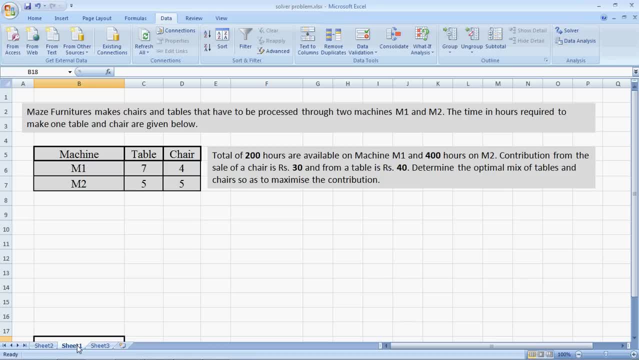 The objective is clear: We need to maximize the contribution. The decision variables are number of tables and chairs to be made, And the constraints are the capacities of machine M1 and M2.. So let's start Initially. I will input the decision variables. 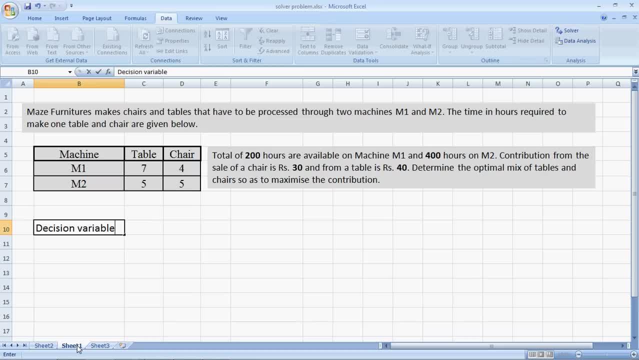 The tables and the chairs. Next come the contribution It has been given to us, that tables make us Rs 40 and chairs make us Rs 30. The total contribution is equals the contribution of one table multiplied by the number of tables, plus the contribution from one chair multiplied by number of chairs. 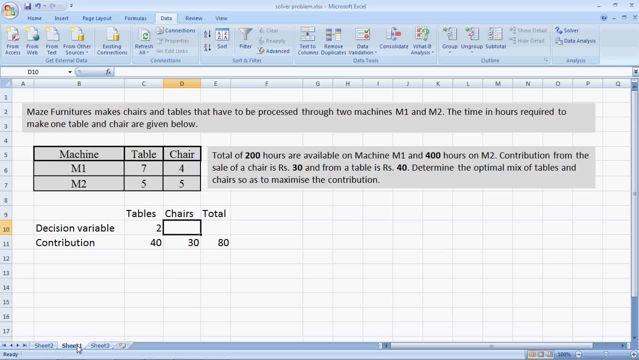 In case I make two tables, I should earn 80.. And if I make three chairs, I need to make 90 more, which should make it 170.. Perfect, Now let's look at the constraints. My first constraint is the capacity of machine M1. 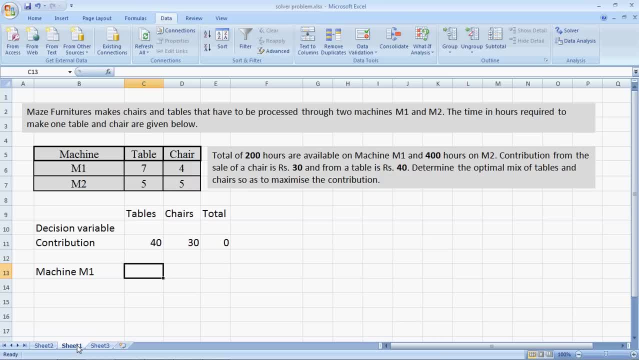 Each table on M1 needs 7 hours and each chair on M1 needs 4 hours. So the total capacity used Equals the time taken by one table multiplied by number of tables, plus the time taken by one chair multiplied by number of chairs. 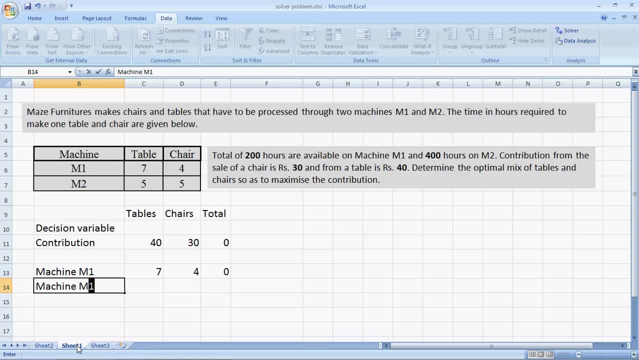 Same thing for machine M2, which is 5 hours per table and 5 hours per chair. We use the same method: Time for one table multiplied by number of tables, plus time for one chair, One chair multiplied by number of chairs. We also need to add the available capacity. 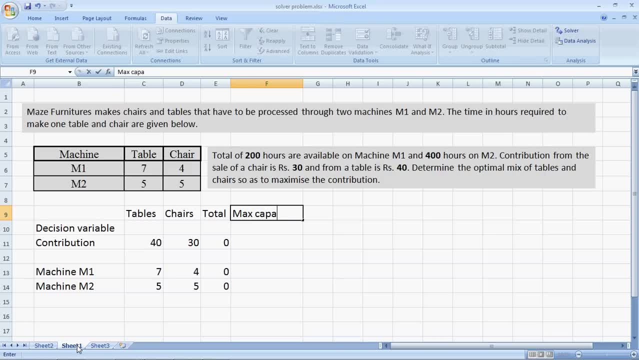 The maximum capacity of the constraints: For M1 it is 200 hours and for M2 it is 400 hours. The formulation has been done. We can go to Solver. The target cell is, of course, the total contribution which has to be maximized. 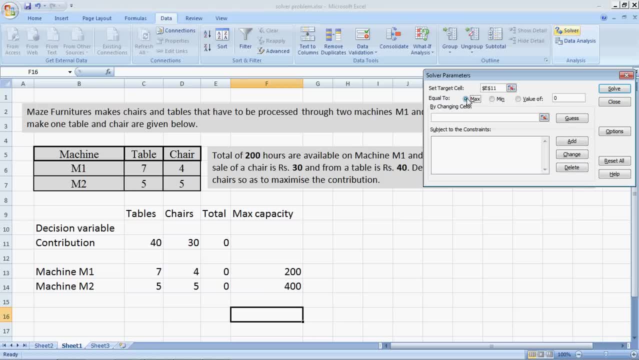 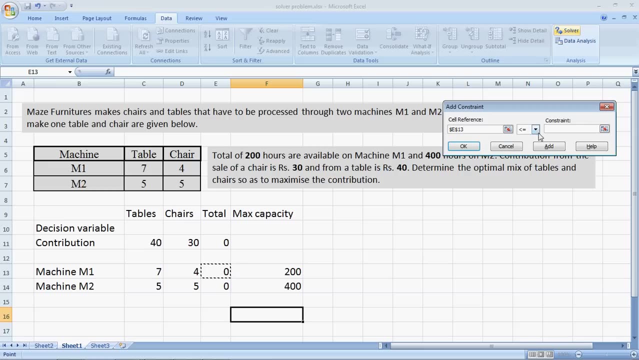 We could have minimized it also. The changing cells are the decision variables. I can change the number of tables and chairs And my constraints are the capacity used in M1, which has to be lesser than the capacity available on M1. We can change this to make it equal to greater than. 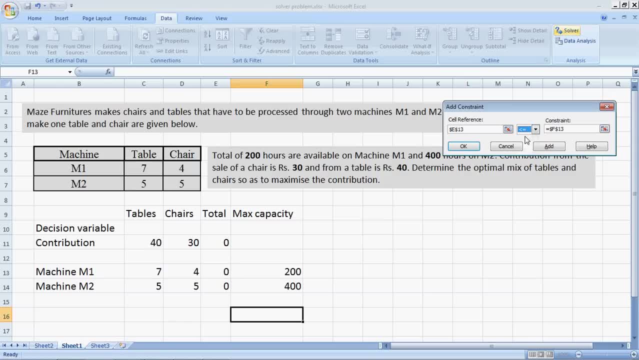 Make it an integer or a binary, But we will stick to less than. We add one more constraint. We say the capacity of M2 has to be less than or equal to the capacity available. We say OK, We go to Options, The Options button. 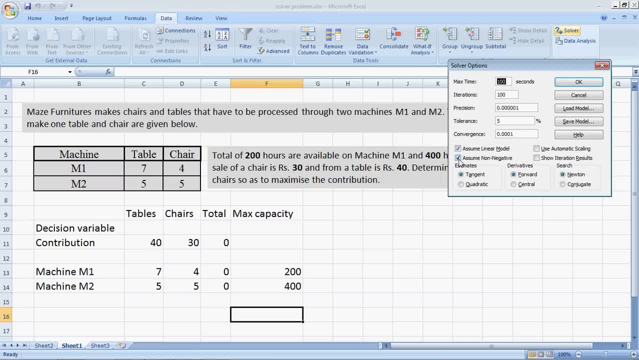 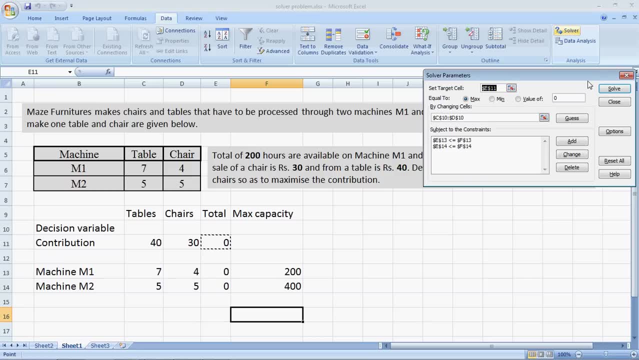 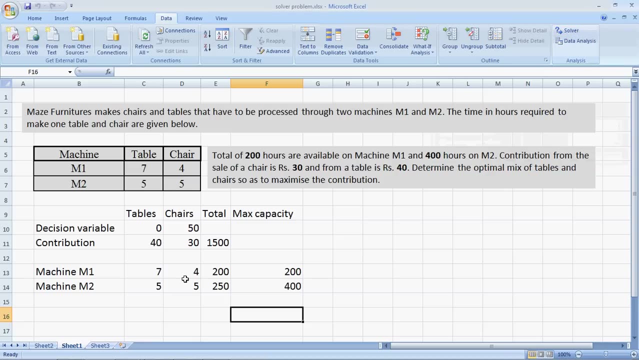 We assume it to be a linear model And we also assume non-negativity- that we cannot make negative tables and negative chairs. OK, Then we leave it to Solver to tell us the best solution. As for Solver, we should make 50 chairs and no tables. 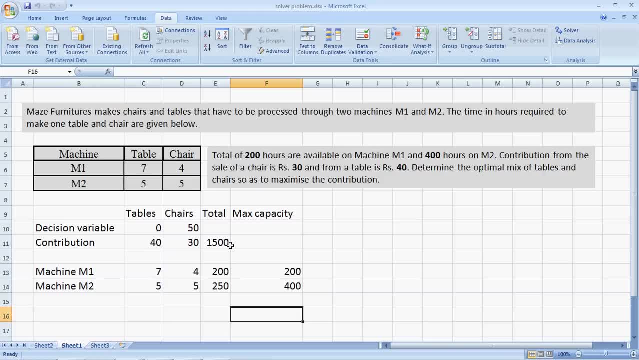 And we will have a contribution of 1500 rupees. We will completely utilize the capacity on machine M1. And we will utilize 250 out of the 400 hours available on machine M2.. That's how simple it is, Thank you. 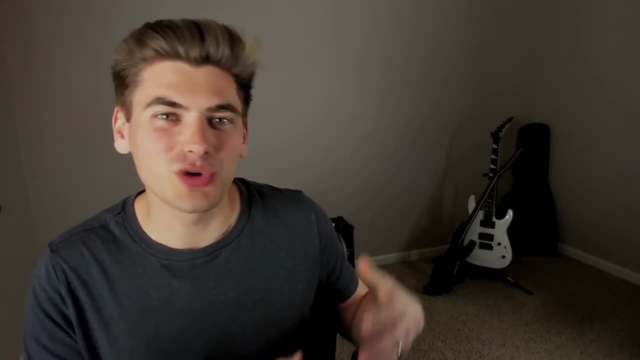 The biggest reason your website feels slow is because your images load like this. It's painful to look at and just makes your website feel incredibly sluggish, even if everything else is blazing fast. That's why, in this video, I'm going to show you how to make. 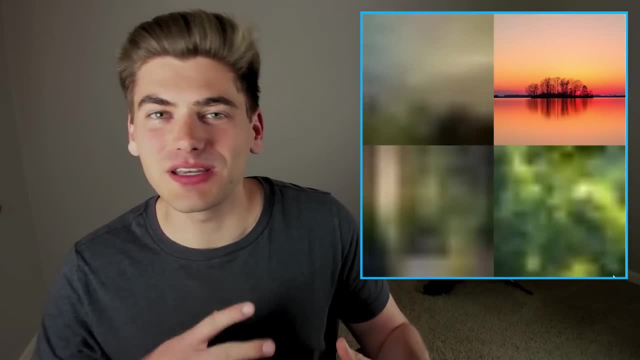 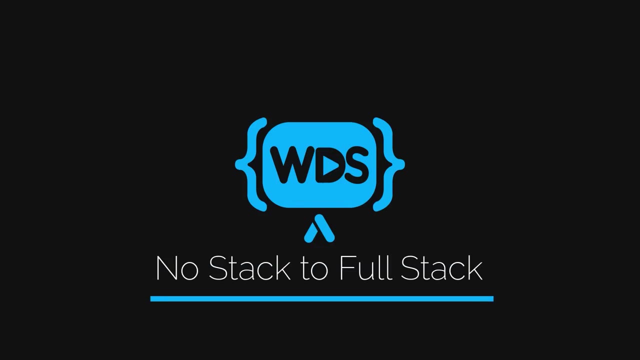 your images load like this instead, As you can see, we got that really nice blurry background. it's going to be lazy loaded and everything is going to be super performant. Welcome back to Web Dev Simplified. My name is Kyle and my job is to simplify the web for you. 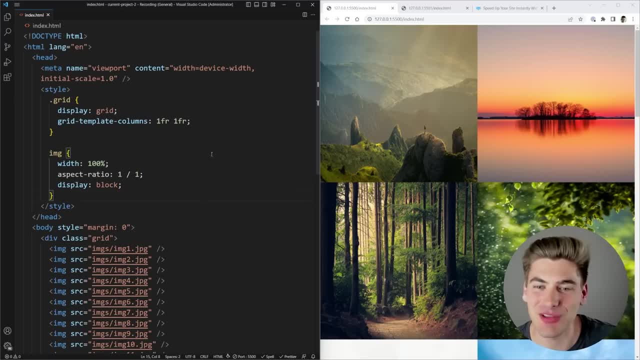 so you can start building your dream project sooner. and today we're going to talk about lazy loading images, as well as getting that blurry loading background that I showed you at the beginning. As you can see here, when I just refresh this page, it looks like everything is incredibly. 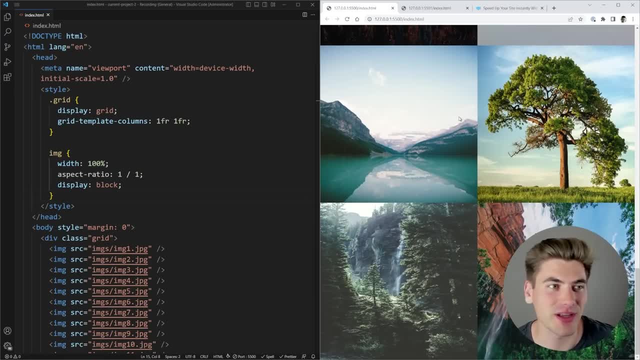 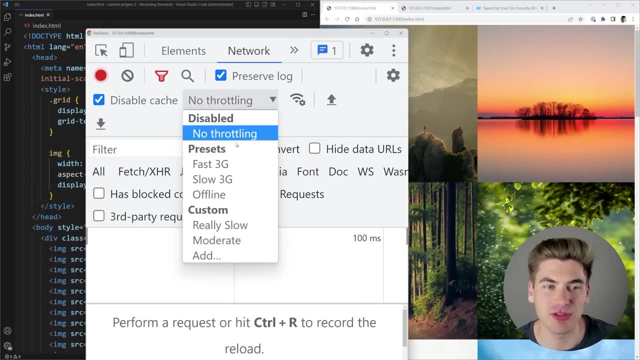 quick and responsive, and that's because my internet speed is incredibly quick and I'm downloading local images. But if I try to emulate what happens on a slower internet connection by coming over to my network tab and I'll just do something like fast 3G, for example, and I'll just 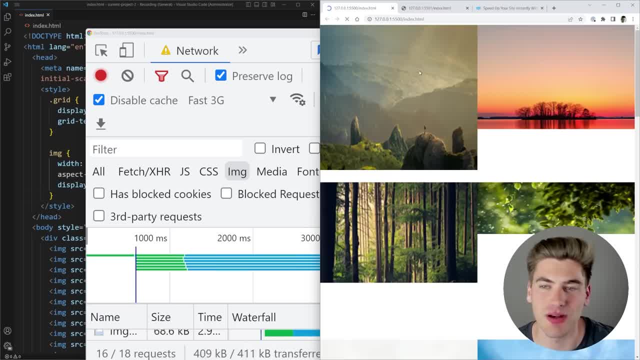 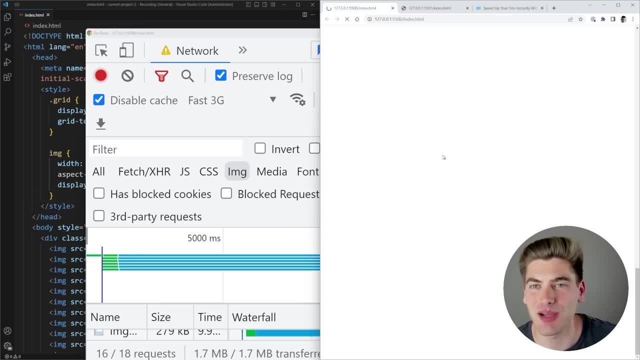 do a refresh on this page, you'll notice that the images load in incredibly slowly, as you can see, and when I scroll down to the bottom the page, all I get is essentially a giant white box, which is obviously not ideal. instead, I would like my images to have this nice little blurry background to them, which 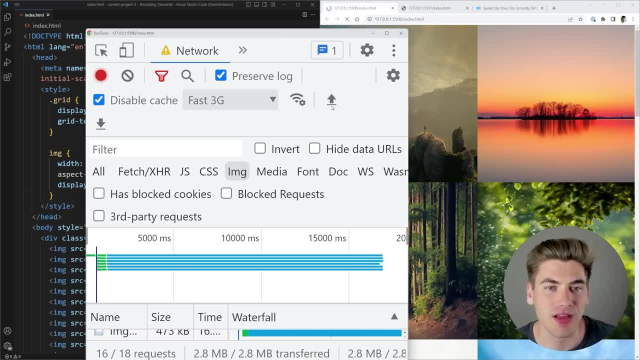 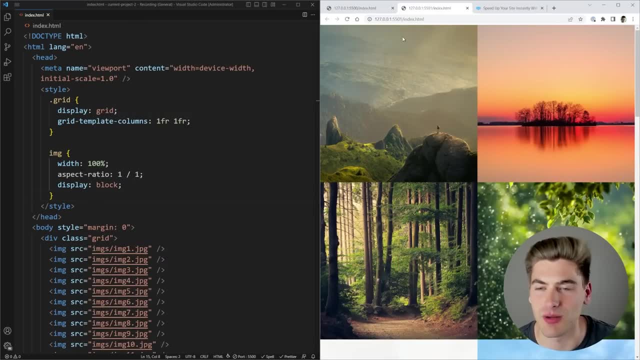 would look a lot better instead of slowly loading in one after the other. Now, if I go over to this other example- this is the final working example. as you can see, when my internet speed is fast, everything refreshes incredibly quickly and it looks quite good. and if I go over and I change,